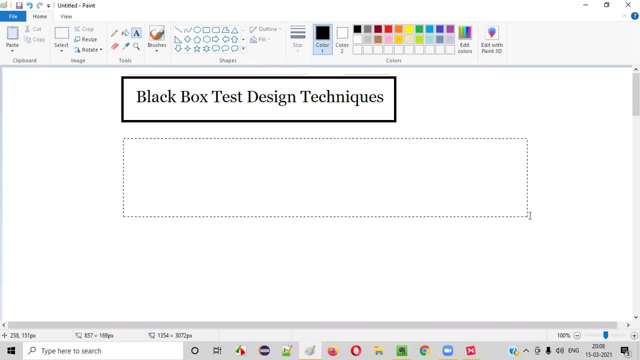 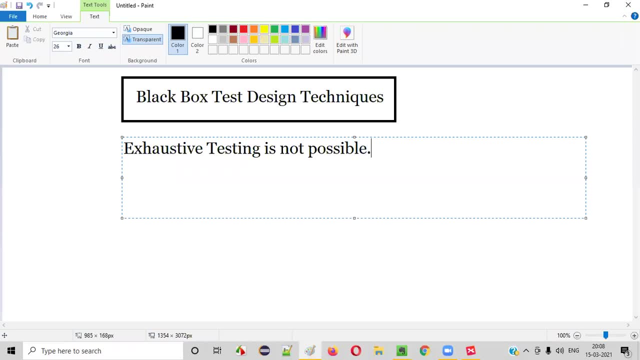 box test design techniques. we have to first understand that exhaustive testing is not possible. Exhaustive testing is not possible. What does it mean, guys? Exhaustive means complete, Complete testing is not possible. Why complete testing is not possible? Let me give an example. 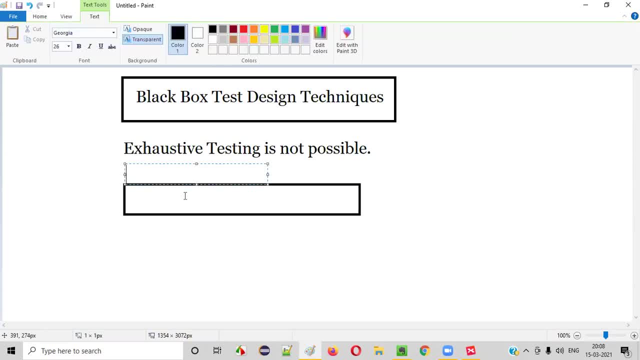 Let's say there is a text box field which can accept the numerical values from 1 to 1 crore. Okay, this text box field can accept the numerical values from 1 to 1 crore guys. so in order to completely test this particular text box field, how many times i need to perform? 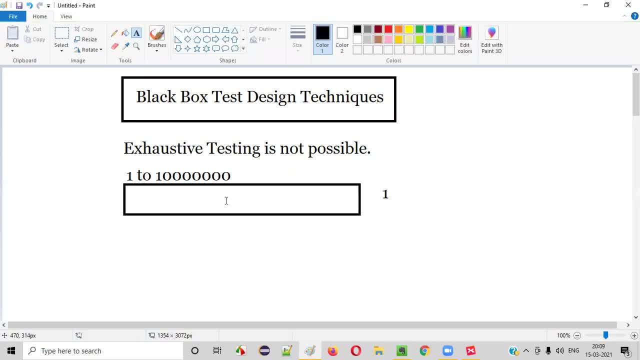 testing guys. initially i have to provide the number one into the text box field and see whether this field is accepting the one value or not. if it is accepting, then i'll enter the next value, that is, two, and see whether the text box field is accepting this two or not. it has to accept. 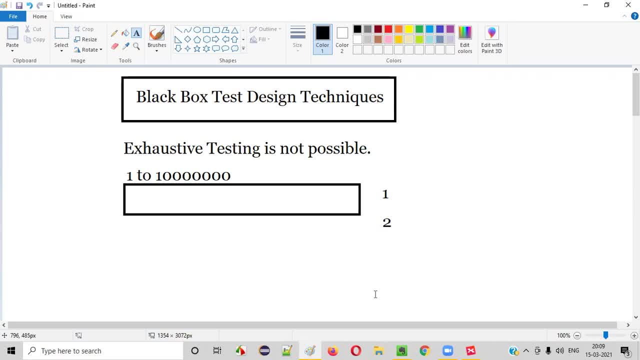 similarly after one, two. i'll keep on going till one crore. how many times i need to perform testing? one crore times guys. starting from one to one crore. i have to perform testing, not only these guys. this particular text box field should only accept the values from one to one crore. that means 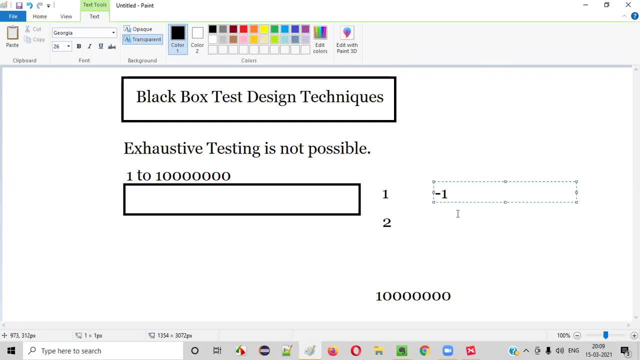 it should not accept the negative values. okay, you should not accept minus one, you should not accept zero, you should not accept minus five. all negative numbers it should not accept here. inputs are endless, guys, it's a infinite. okay, infinite negative values are possible here. okay, that can be entered into this text box field. not only these negative values, guys, but also. 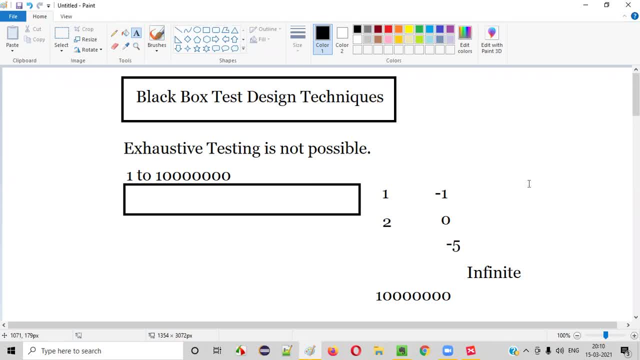 we have to also see whether this particular text box field is not accepting the other type of surprising values, like which involves: some alphabets- okay, or some symbols- okay, some symbols. it should not accept symbols. also, it should only accept the numerical values from one to one crore. apart from that, it should not accept everything. that means, guys, in order to 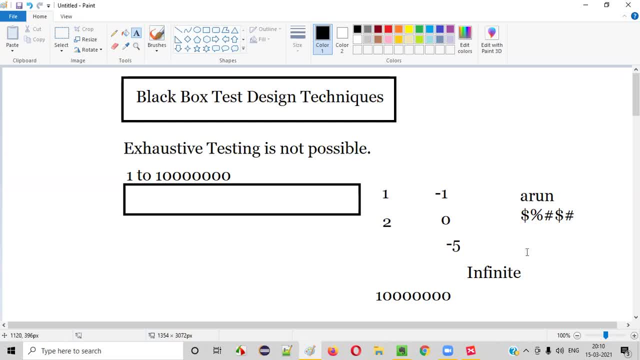 completely test this particular text box field? how many times i need to perform testing? infinite inputs are possible, guys. infinite times are possible, okay, so which, uh, after spending good number of years also, you'll not be able to complete, just for testing the simple xbox field. exhaustive testing is not possible, then, then how to be sure that this particular text box field is? 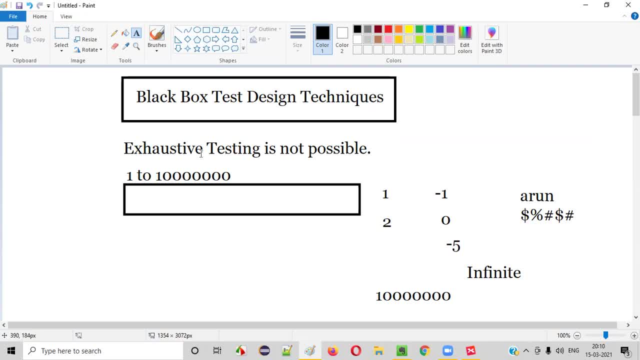 working as per the expectations or not. as exhaustive testing is not possible, how, how can you confirm, as a tester, that this text box field is working fine or not? we have to use something known as black box test design techniques, guys. okay, since exhaustive testing is not possible, we have to use this, uh, black box test design techniques to filter out. 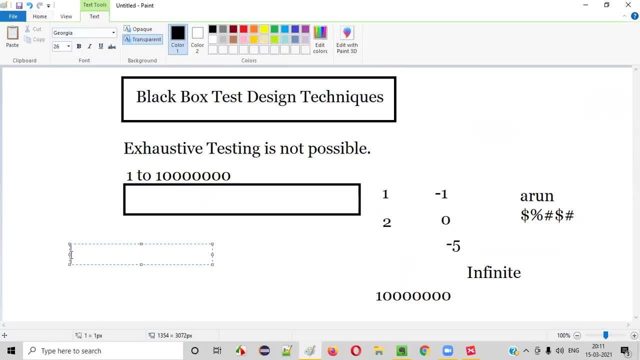 these inputs, why we have to use this test design techniques in order to filter out the inputs. how many inputs are possible here? infinite. so from that infinite inputs, we have to filter them to around max 10 guys. max 10 inputs, generally okay, averagely speaking, max. 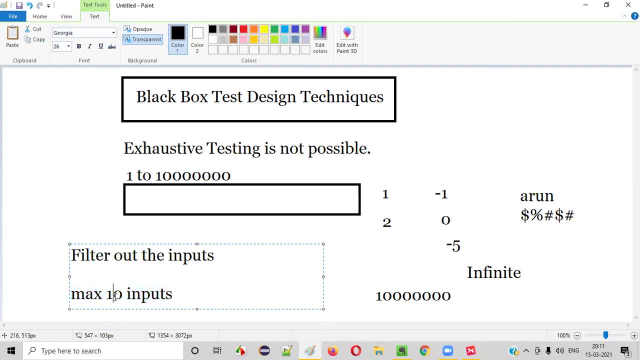 10 inputs. sometimes three, four, five, six. okay, maximum 10 inputs. we have to concise all these infinite possible inputs into just maximum 10 inputs, guys. okay, so just by testing this particular text box field with this maximum 10 inputs, we should be done with the testing. so how to filter? 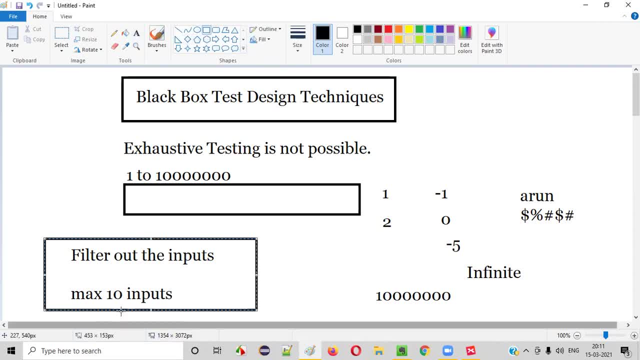 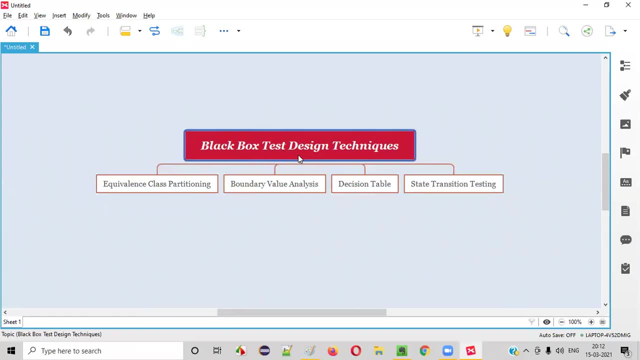 out the inputs from the maximum infinite to the maximum 10 inputs or something, by using this test design techniques. guys, there are several black box test design techniques. let me show you. as you can see here, there are mainly four types of black box test design techniques like equivalence, class partitioning, ecp, boundary value analysis, bva decision table. 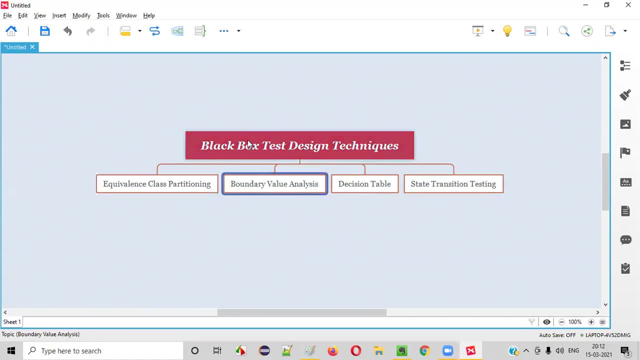 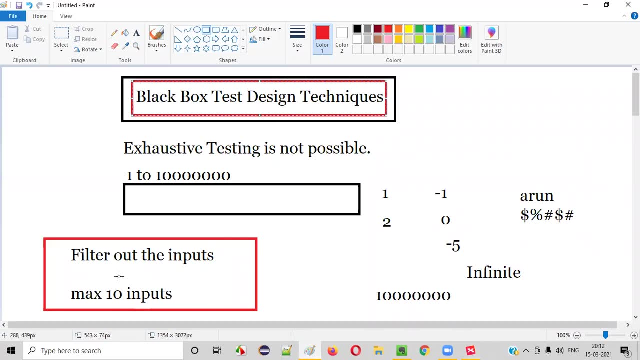 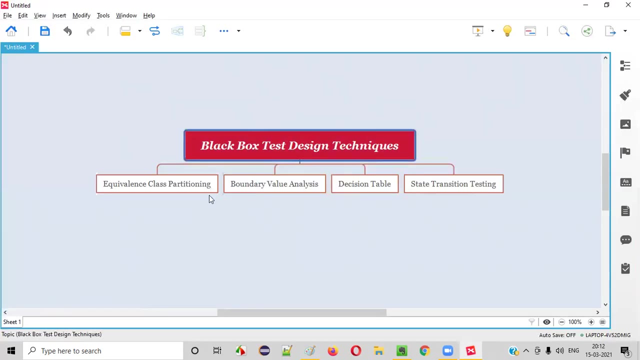 and straight transition testing. these are the four major black box test design techniques which we have to use for filtering out this infinite number of input possibilities to just max 10 inputs and test this particular text box and complete this test design techniques testing. okay, which is kind of practical, right, practically speaking, this is possible, but infinite. 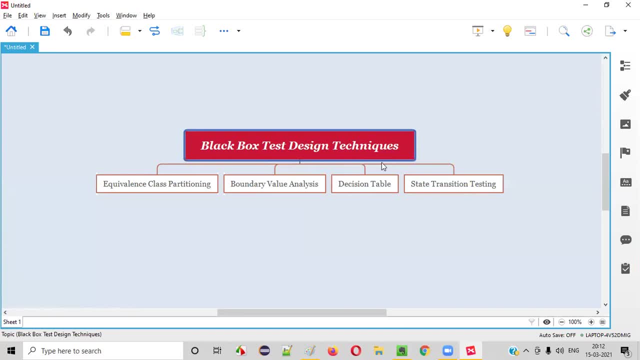 testing is not possible, so we have to apply this black box test design techniques to filter out the inputs to maximum 10 inputs or something okay, using this different test design techniques, i will be explaining guys in detail, like how to apply this equivalence class partitioning test. 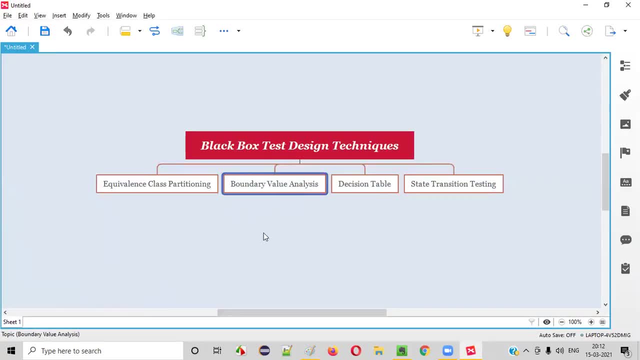 design technique for filtering out the inputs. how to apply this boundary value analysis. test design techniques to filter out the inputs. decision table test design techniques to filter out the inputs and state transition testing. test design technique to filter out the inputs and derive the appropriate test cases using this guys test design. it's here the name itself is speaking about test. 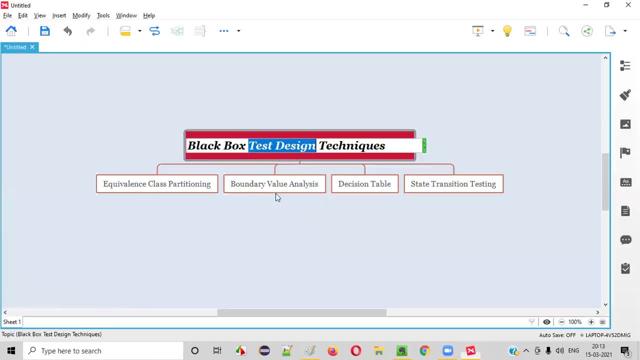 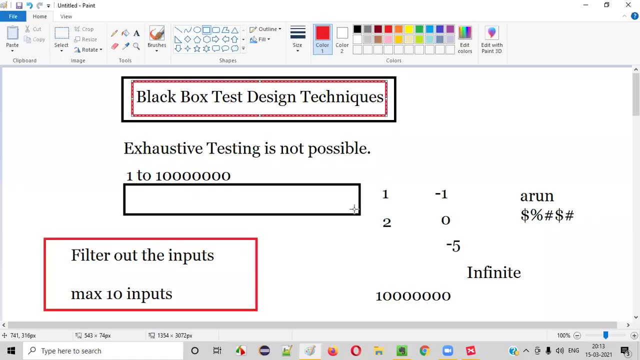 design. that means creation of the tests. okay, here inputs are related to the test test cases. guys, okay, using this different black box test design techniques, we can create the test cases. okay, instead of infinite number of test cases. we can concise them to simple: okay, general list number of test cases. we can concise them to simple: okay, general list number of test cases. 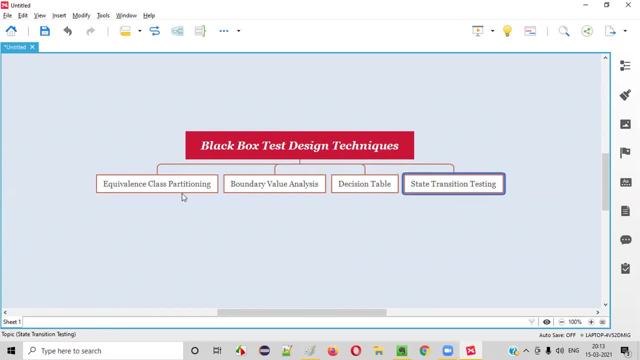 we can concise them to simple: okay, general list: number of test cases which are which are effective kind of test cases: okay, using this design techniques, we can simply design effective test designs. okay, test cases instead of a lot of possibilities- okay, fine. so in the upcoming sessions, guys, i will take separate sessions for each and every test design technique that i am. 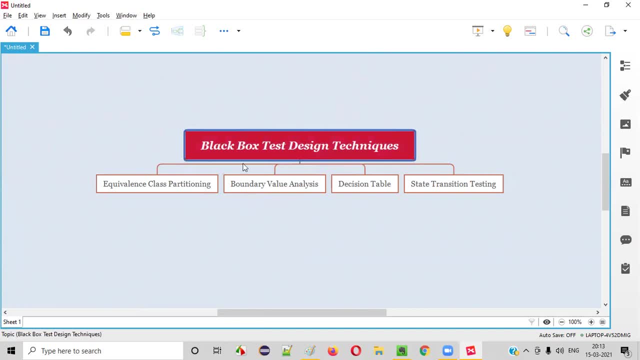 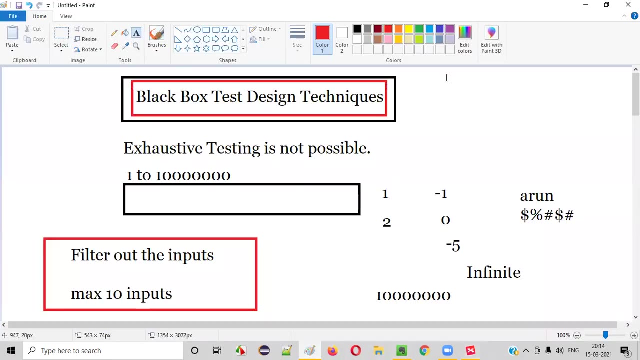 representing here. fine, so, guys, this black box test design techniques are also known as: okay, other people, or there are different names. guys, there are different names. there are different names for this black box test design techniques. so what are the other names we have? the other names are specification based. we can also call this black box test design techniques, as 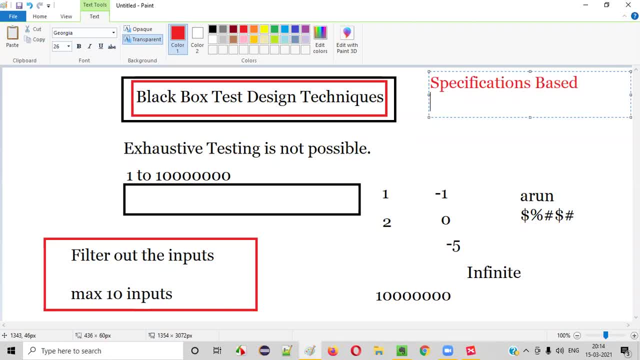 specifications based test design techniques. this is one of the other name people call black box design techniques, with another other name also here and there. so instead of calling them black box test design techniques, few people will call them specifications based test design techniques and some other people will be calling them behavioral, behavioral testing techniques. 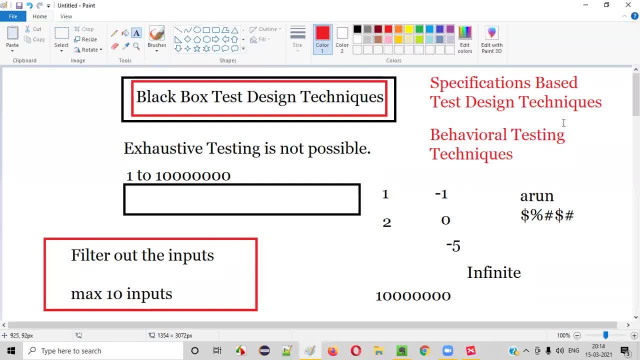 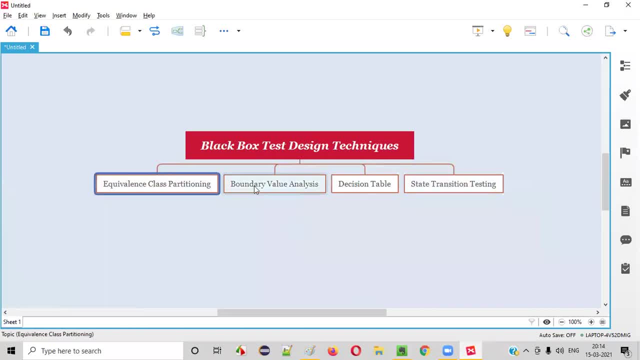 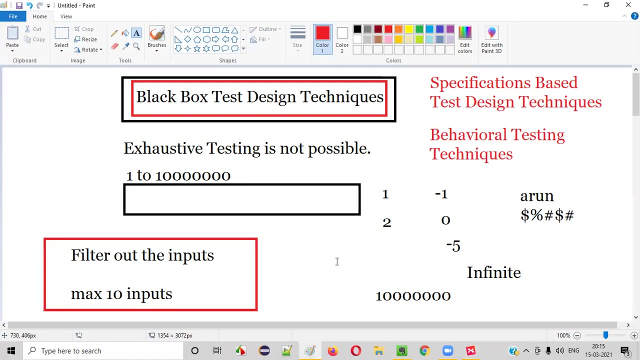 everything is same, guys. okay, either you call them black boxes and techniques, or specification based design techniques, or behavioral testing techniques. these are the four major ones. okay, these are the four major test design techniques, guys, which we can use for effective test designing by filtering out the number of infinite inputs to the just maximum 10 inputs. okay, maximum 10 inputs. 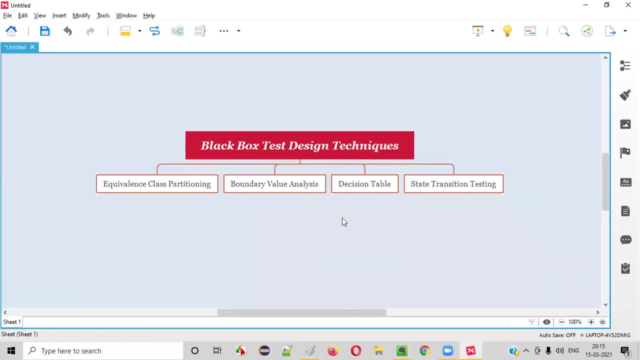 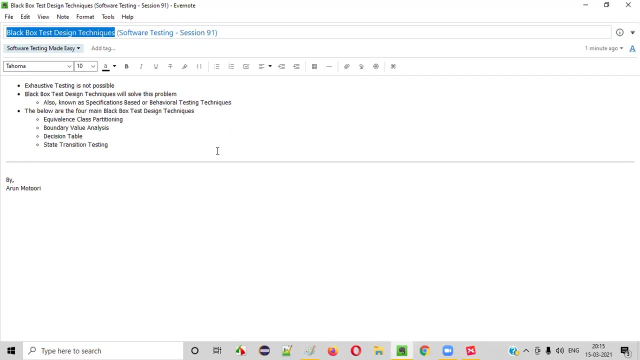 in average, guys, generally maximum 10 inputs. it will come to fine. so hope, guys, you understood what exactly are this black box test design techniques and what is their purpose. so that's it, guys. see you in the next session. thank you bye.